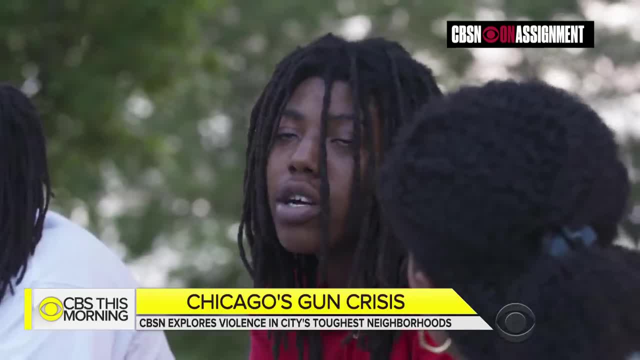 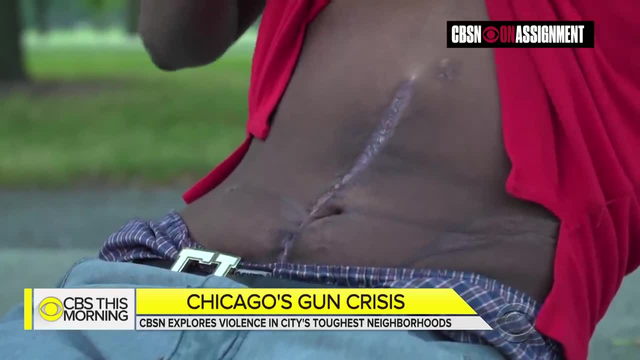 I got shot twice and I thought I'd been gone, but I'm still here. so that's God, I know that's with me. so this here, It's hell on earth. It's hell on earth. Yeah, it's hell on earth. 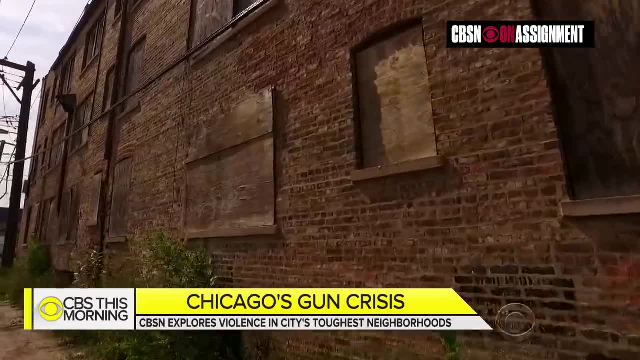 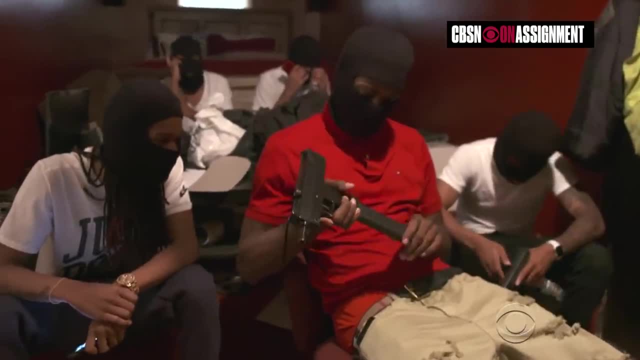 The problem we heard and saw over and over again was guns. We make sure ourselves secure, We make sure ourselves safe. CBS News gained access to several crews on Chicago's south side. Yeah, man, this is a Mac right here. man, That's 50 shots, man. 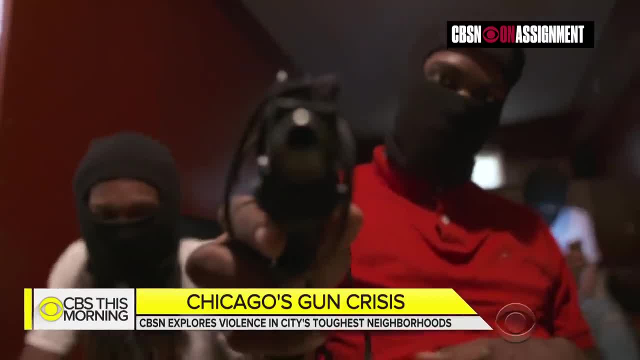 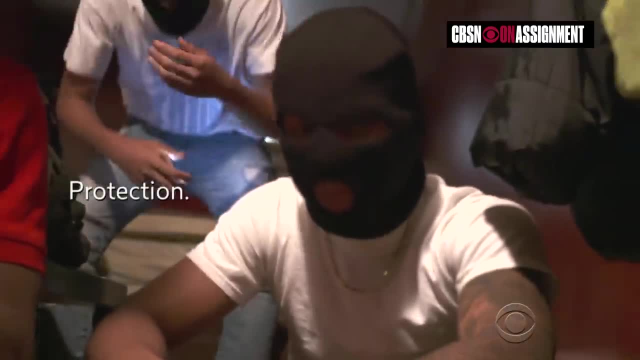 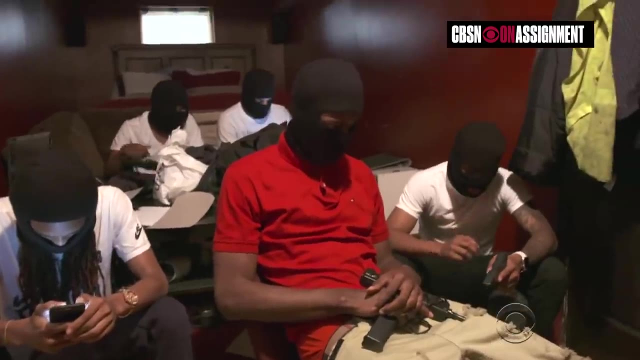 That's a Mac-10, a semi-automatic weapon, originally designed for military use and illegal in Chicago. So why do you need guns? Gun is firepower Protects. It's dangerous out here. This south side crew is affiliated with the group the Titanic Stones. 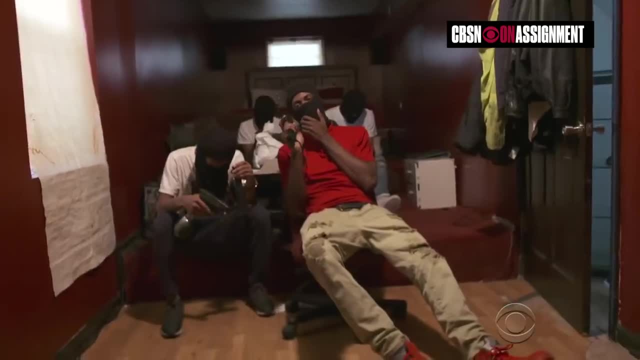 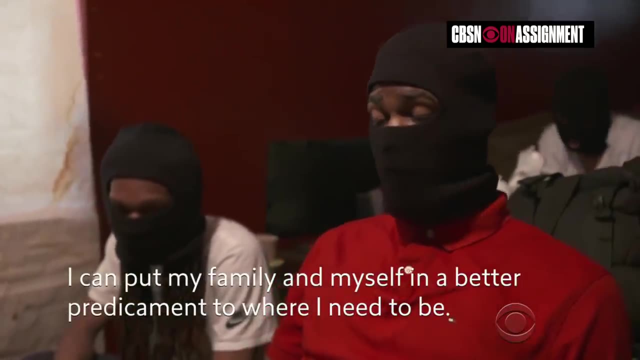 They cover their faces to conceal their identities. They actually told us they hate guns. I'm in with this gun. I'm just doing this for survival, bro, until I can put my family and myself in a better predicament to where I need to be. We're just trying to keep ourselves protected. 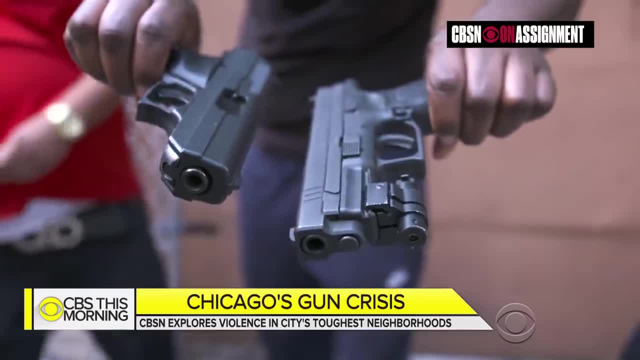 Many guys told us they'd rather risk the police catching them with a gun than have their lives in danger, And that's why some of their rival find them without one. Where do you get a gun like this? Where did you get this gun? 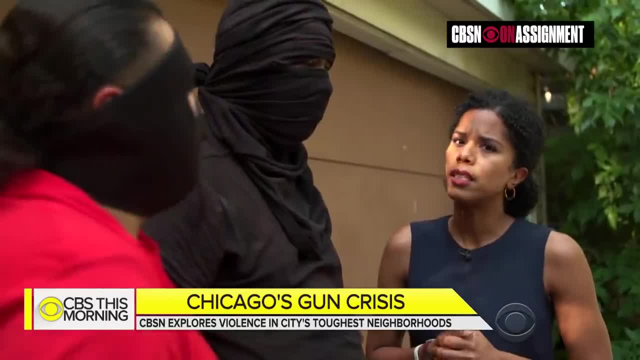 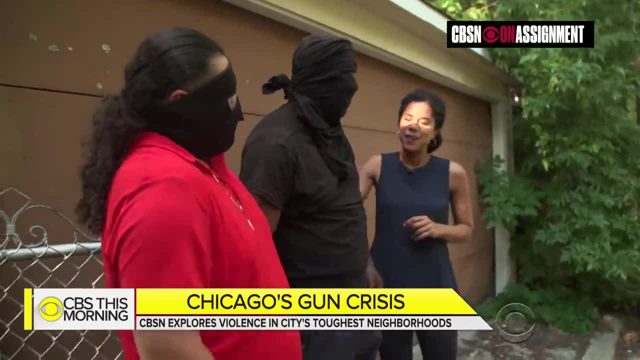 Off the streets, people sell them. How easy is it for someone to get a gun? That easy? You want one? No, Just like that. That's how easy it is And it's worth it for you to keep this gun. 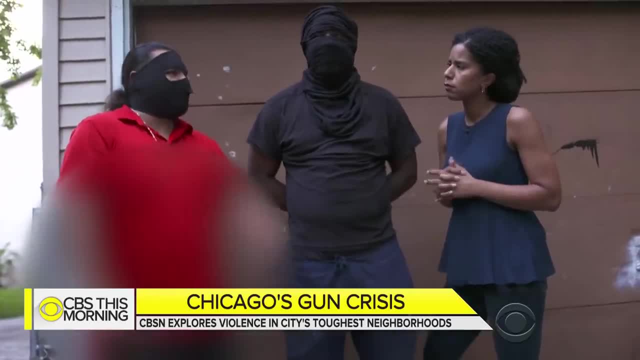 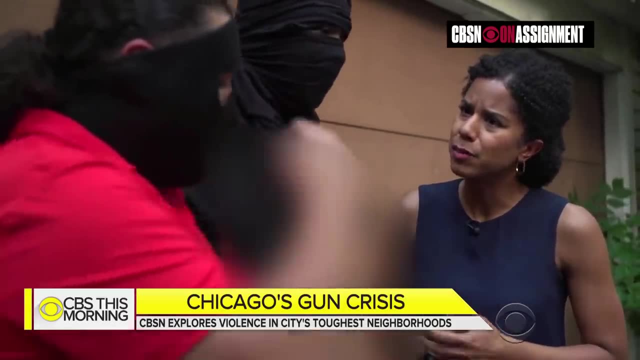 We're felons. you know what I'm saying. See how many people. you see how many people. The cops don't give a f*** about us. But with so many innocent people dying by these bullets, is it worth it? No, 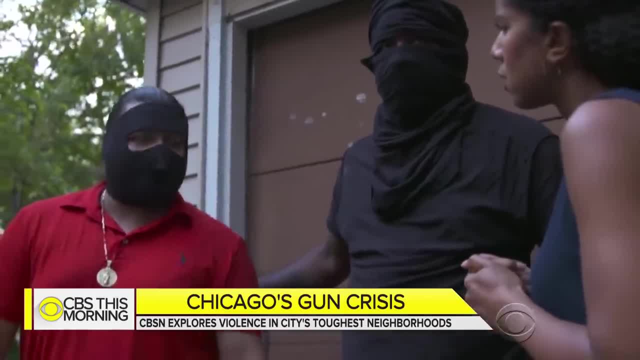 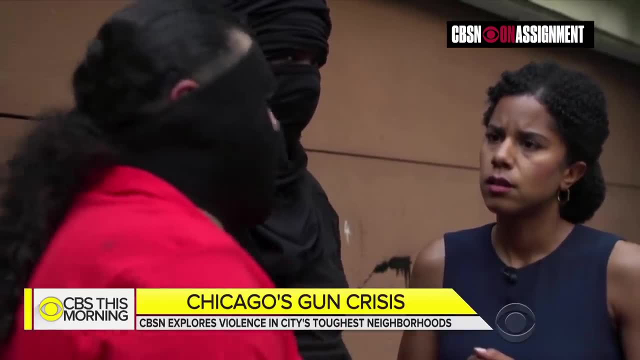 I mean No, In the end it ain't worth it. boy, You got dumb a*****. you want to go pull a drill, a drive-by- you know what I'm saying? And some innocent little sister gets shot. Now guess what? them and them guys are coming back. 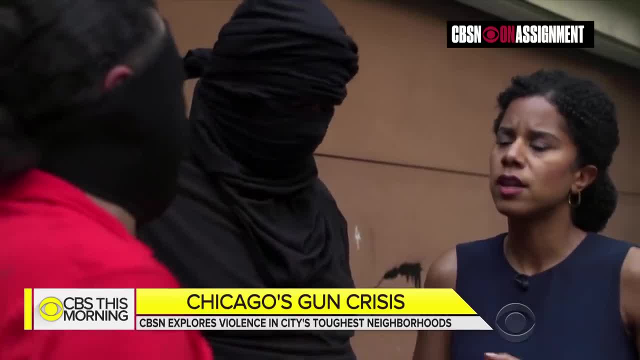 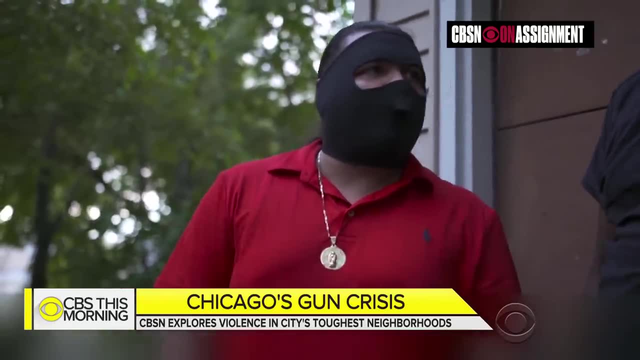 And that's how the confrontation is just going to keep going. Why not just put the guns down? Put the guns down. Well, it probably will happen, Maybe in the near future, just no time. right now, you know, I don't want to put my gun down. 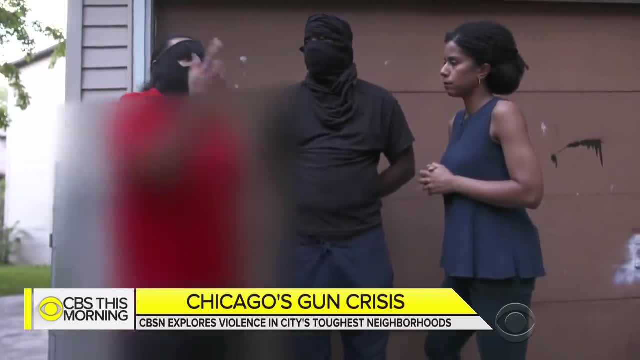 Nine times out of ten the innocent ones getting hurt. you know what I'm saying. If they do come shooting right now, we probably don't even get shot, And we got guns. You might get shot. That's how f***ed up it is, you know.